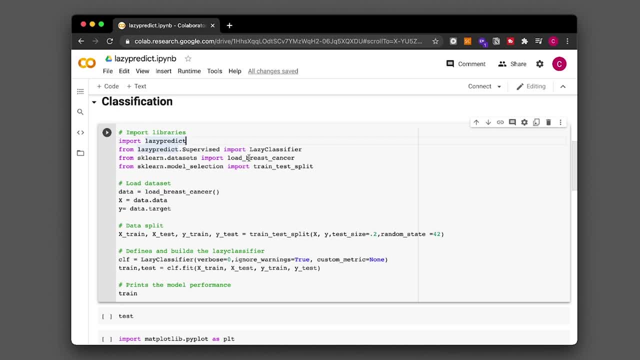 classification, and then we're going to be using the breast cancer data set, so we're going to be importing it directly from the sklearn library. and then we're also going to be importing the train test split in order to build the Lacey Predict library, So we're going to be importing. 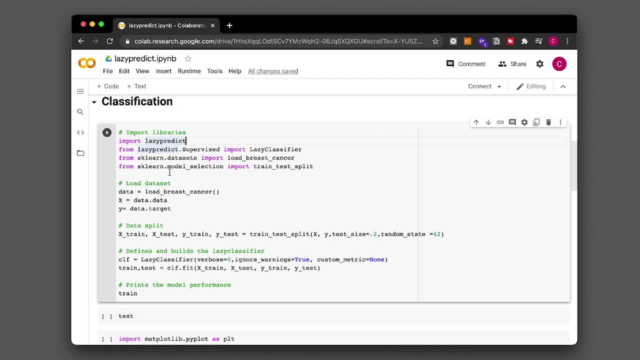 perform data splitting, also from the scikit-learn library. In this blocks of code we're going to be importing the data of the breast cancer using the load breast cancer function. Then we're going to be assigning the datadata to the x variable, And so the datadata is essentially going to be. 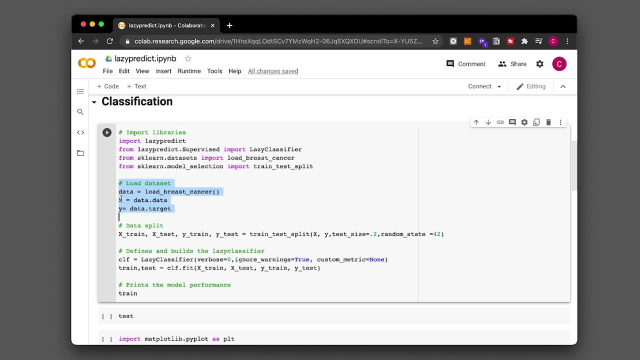 comprised of the x data matrix, And then we're going to be assigning the datatarget to the y variable. Then we're going to be performing data splitting using the 80: 20 split ratio, and a random state will be set to 42. And now we're going to be assigning the Lacey classifier to the CLF. 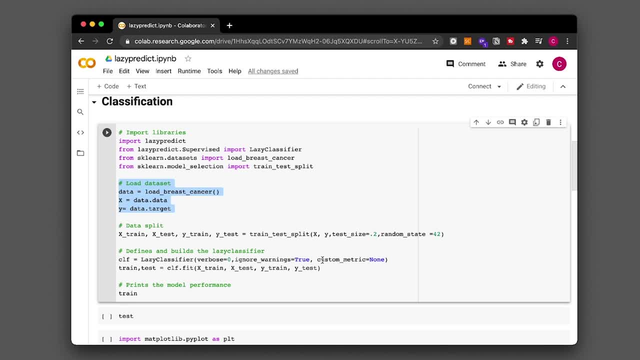 variable, And so the input arguments here were set according to the example provided on the GitHub of the Lacey predict library. And then we're going to be building the models by using the CLF dot fit function And then as import arguments we'll be assigning the x train, x test, y train, y test, And that will 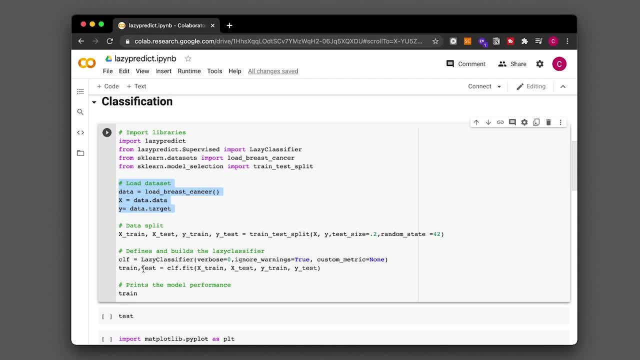 be assigned at the same time to the train and the test variables. So it will essentially be assigning the performance data or the model performance of the training set, and then it will be assigning it to the train variable And then the model performance for the testing set. 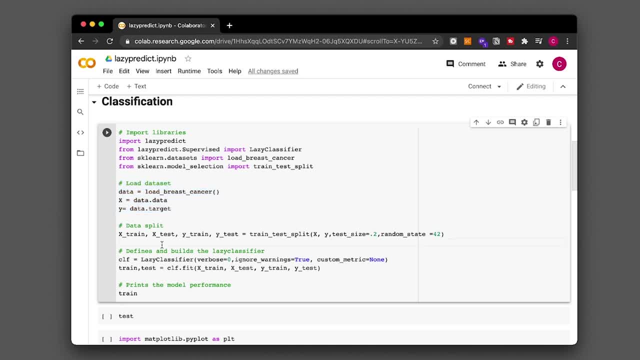 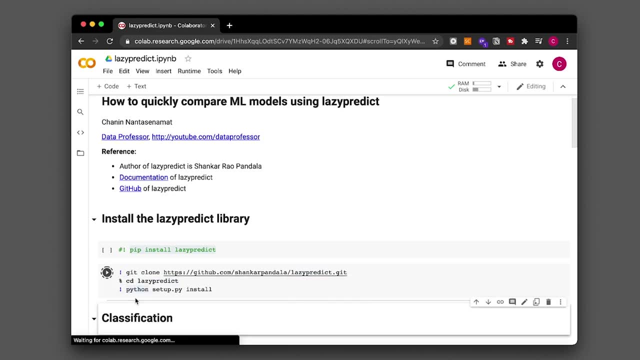 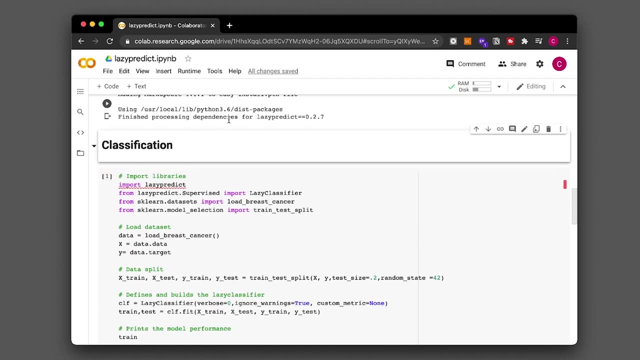 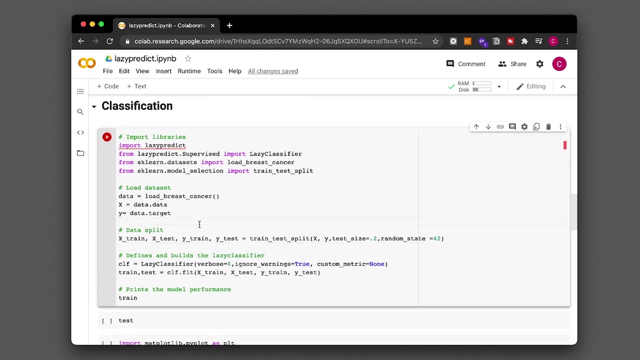 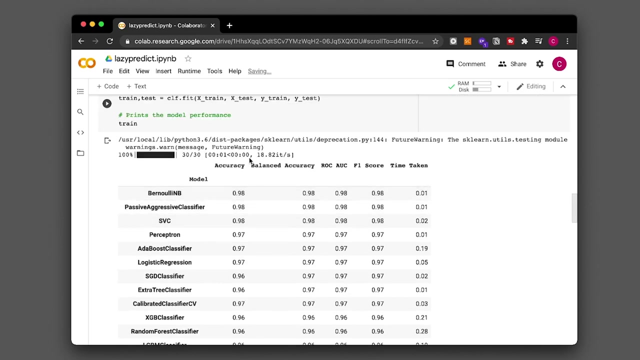 will be assigned to the test variable. Okay, so let's run the cells, Alright, and so we have already installed the Lacey predict library from the GitHub, And let's go ahead and run the classification code cell here, And so it will be building 30 models and the performance will be provided. 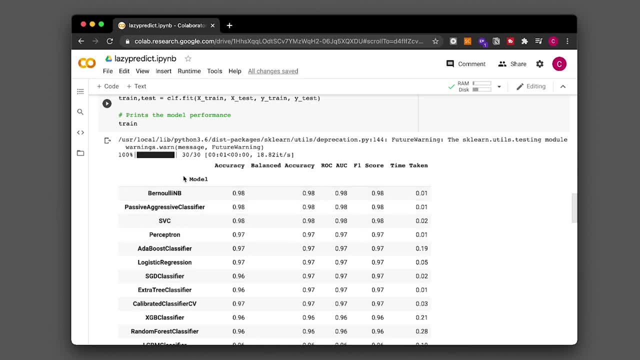 in this data frame. So we're going to be having the first column here, which is also the index of this data frame, to be the name of the machine learning models using the different algorithms of the 30 algorithms. we can see the model performance in the following columns: 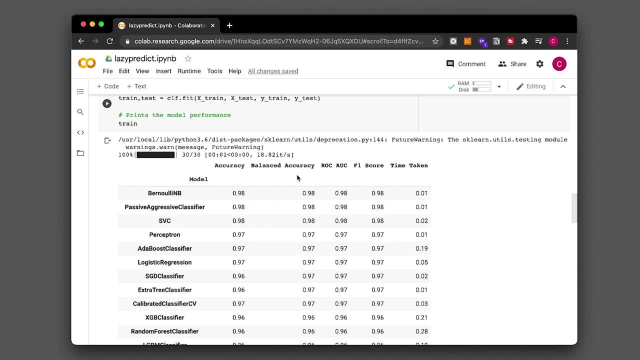 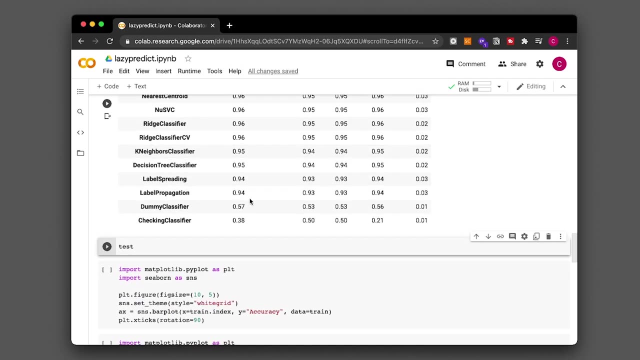 comprising of the accuracy, balanced accuracy, the area under the curve, ROC F1 score and also the time taken to build the model. So let's have a look here. So the model performance are pretty good, mostly 90%. And let's have a look at the test. 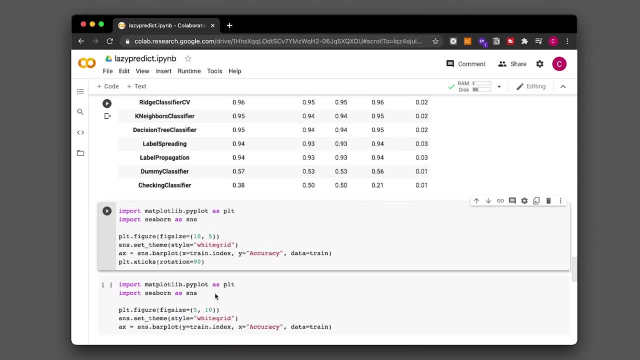 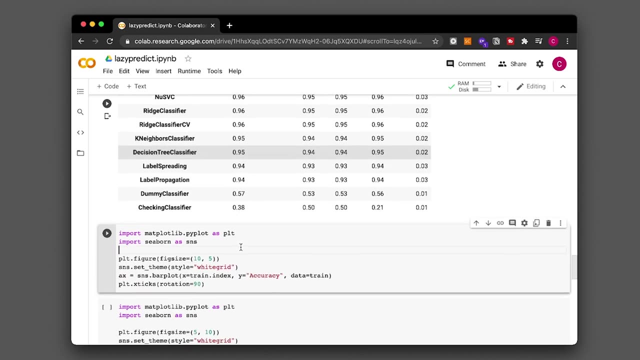 So quite comparable, And so let's have a look at the data visualization. So we're going to be making a bar plot of the machine learning methods and also the accuracy, And then we're going to be showing it. So let's have a look here. 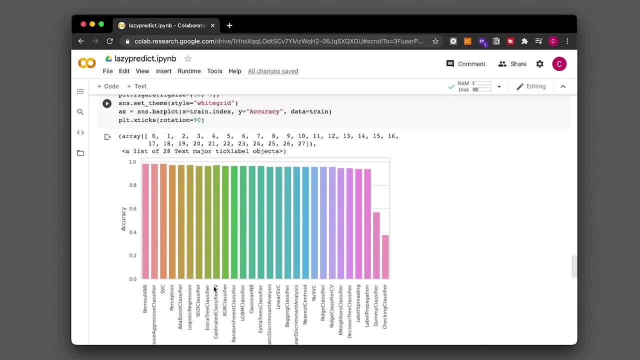 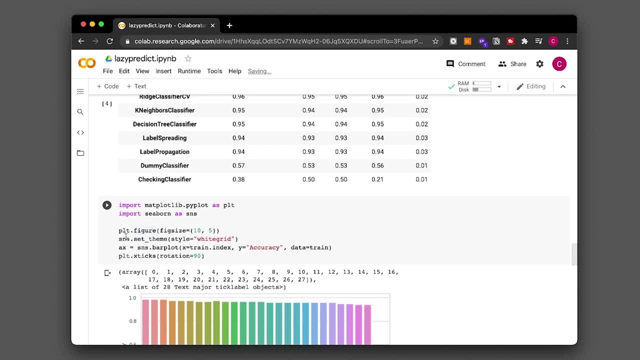 And so in the x axis you'll be seeing the names of the classifiers, And on the y axis you'll be seeing the accuracy. And so here we're importing the necessary libraries, matplotlib and seaborn. And so seaborn will be used for making the plots, and the matplotlib will be used for adjusting the. 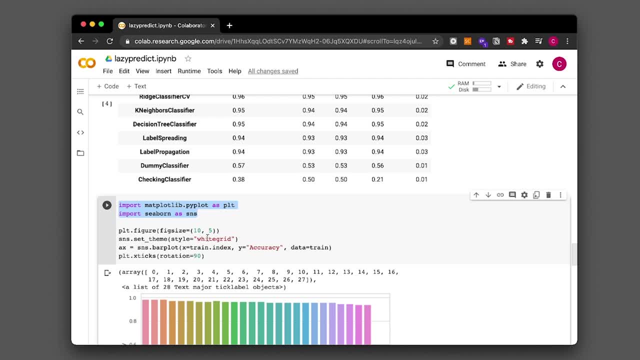 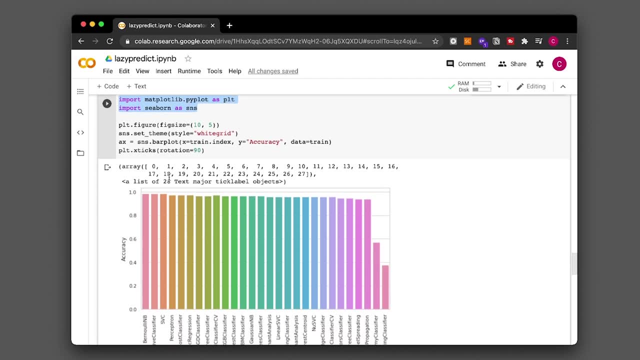 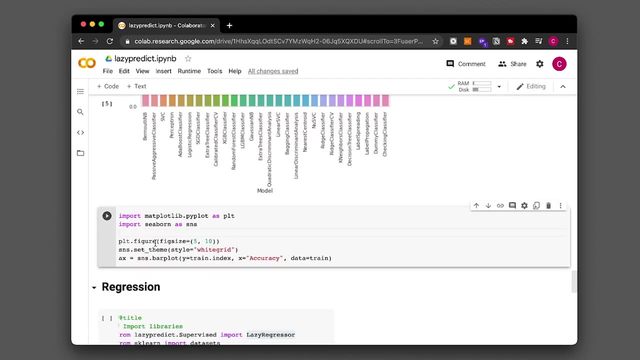 axis label, rotating it and also making it having a white background, as well as adjusting the figure size as well. And so here we're using the bar plot function of the seaborn package And let's run this as well, And so this one will be the vertical version. 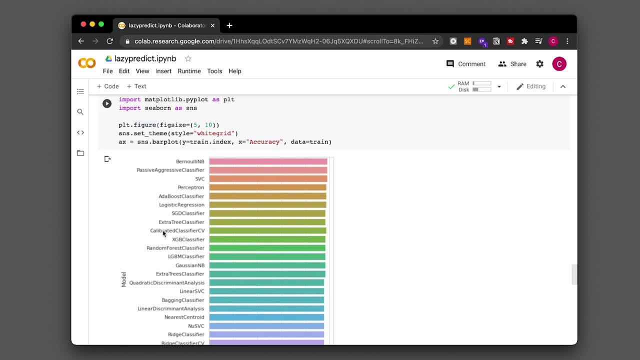 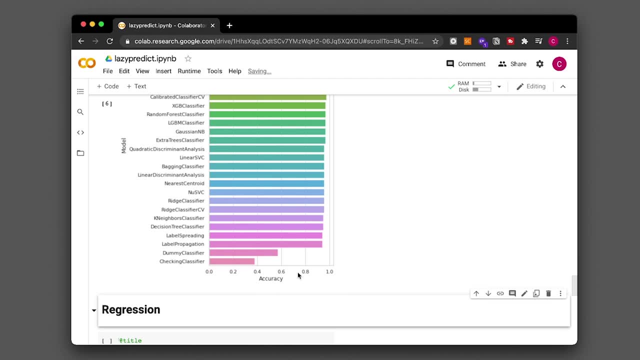 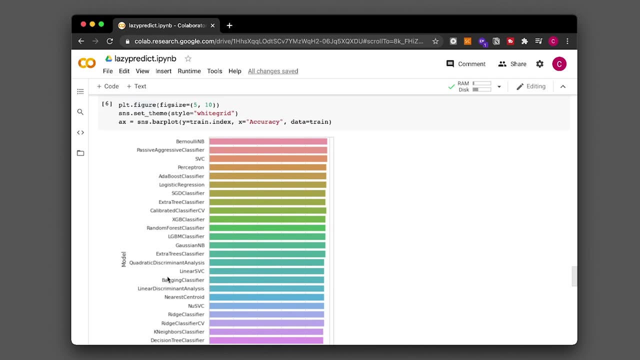 So we're switching and then we're displaying the names of the models in the y axis, And on the x axis we're showing the accuracy value, And so this might be a bit easier to read the name of the classifier, instead of having to tilt our head to read it as in the above one. 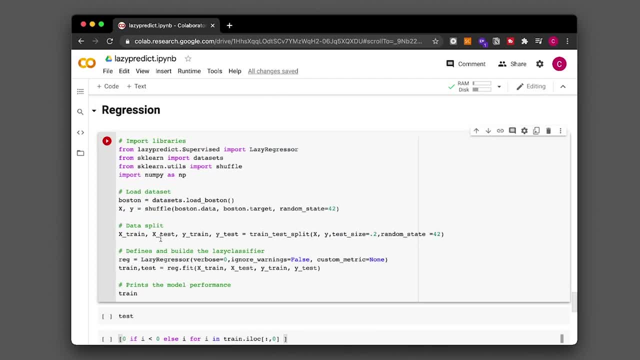 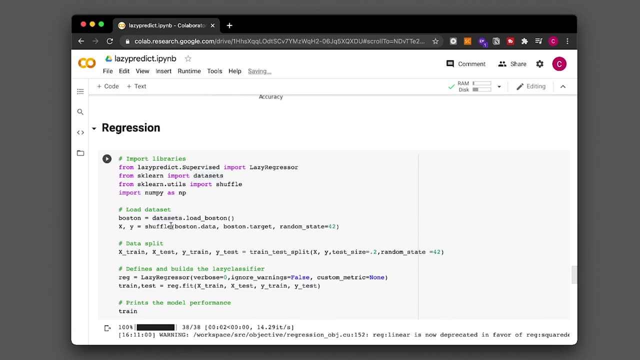 Okay, Okay. so now we're going to be building the regression models. Let's run the cell. So, essentially, we're doing the same thing: we're going to be importing the necessary libraries, we're going to be loading up the data set And here we're going to be using the housing. 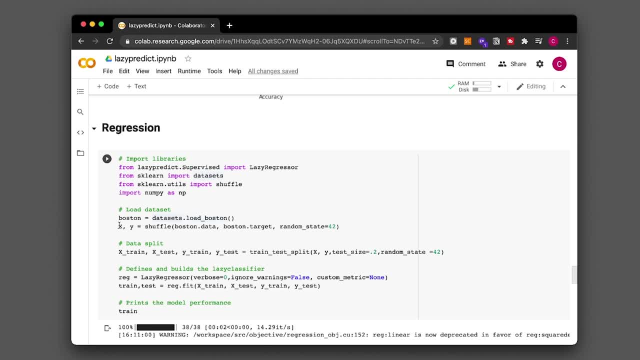 data set of Boston and then we're assigning it to x- y variables. But before doing that, we're also doing the shuffling of the data And we're using a random seed number of 42, we're going to be splitting the data into the training and testing subset and using the 8020 split ratio. 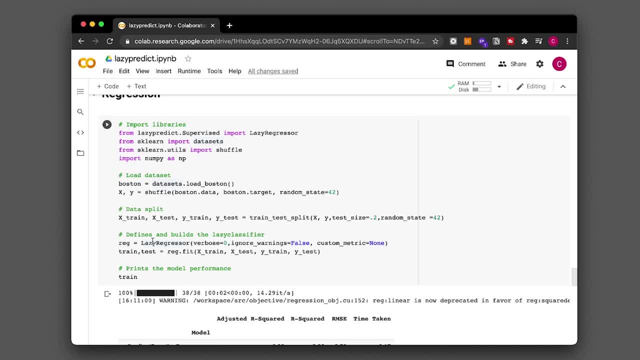 then we're going to be building the regression model using the lazy regressor function, And then we're going to be using the default input arguments provided by the examples on the GitHub of the lazy predict library and then assigning it to the reg variable. And then we're going to 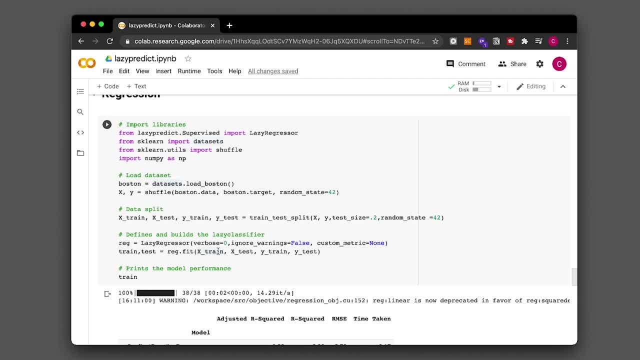 be building the model using reg dot fit. input argument will be X train, X test, y train, y test, And then we're going to be outputting the model performance into the train and the test variables. So they're essentially data frames comprising of the: 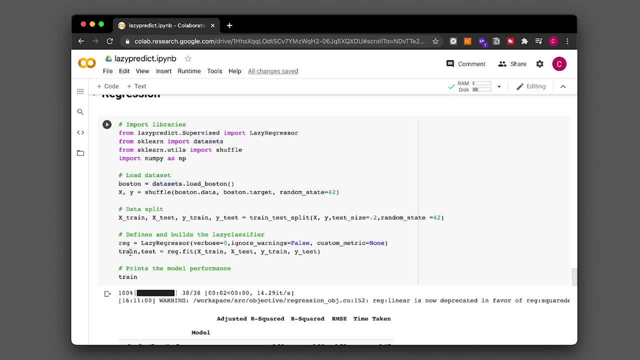 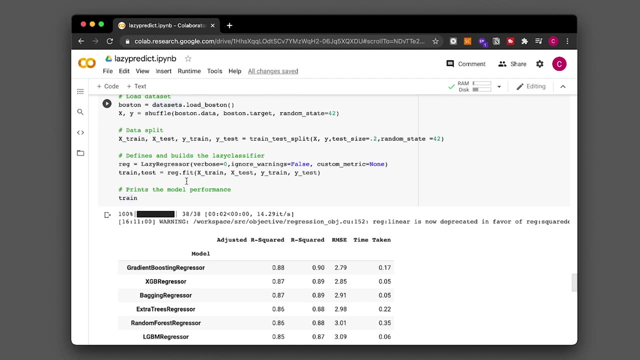 model performance of the training sets and also the testing sets or the two subsets that we have already split it in the above procedure here, And so let's build the model, which we have already did, And we're going to be printing out the model performance of the training subset or 80% subset. 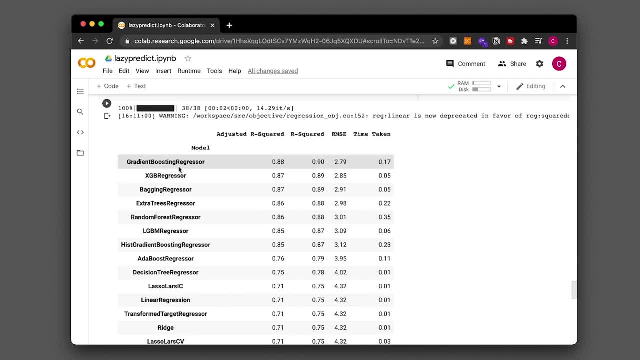 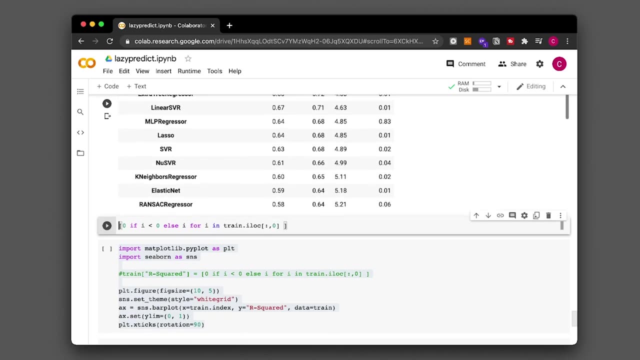 And so here we see that the best model is the in boosting regressor and adjusted r squared of 0.88 and r squared value of 0.9.. Okay, and so let's have a look at the test set. Roughly the same. 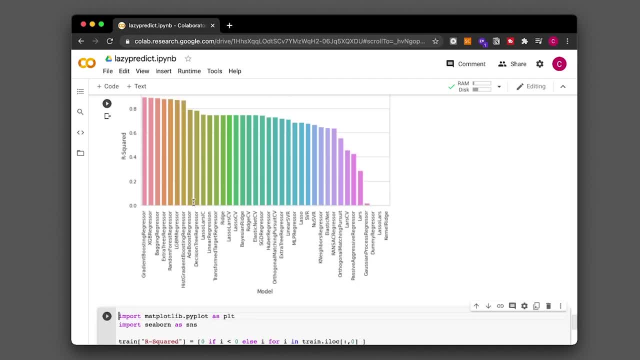 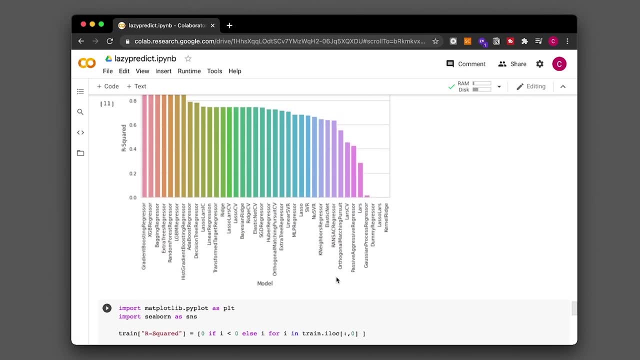 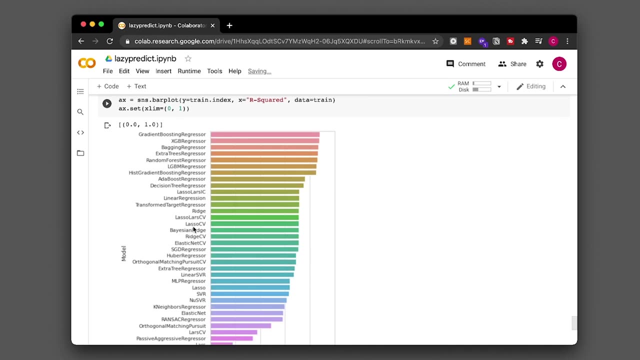 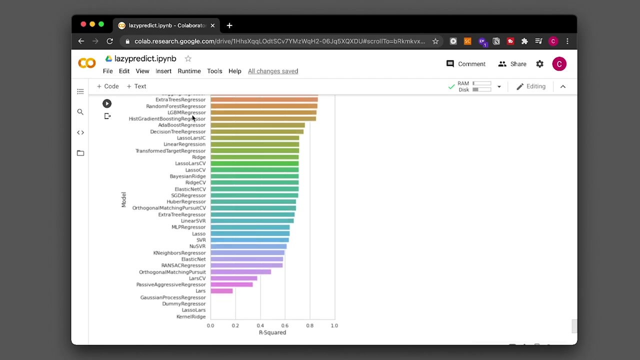 And so let's run the plot here. Okay, So similar representation shown above, The tilted version and also the vertical version. So this is a great way to quickly build several machine learning models using only a few lines of code. And so the thing is, if you have to manually code all of these 30 classifiers, 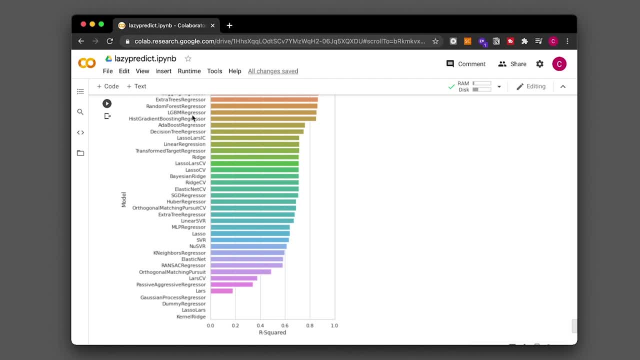 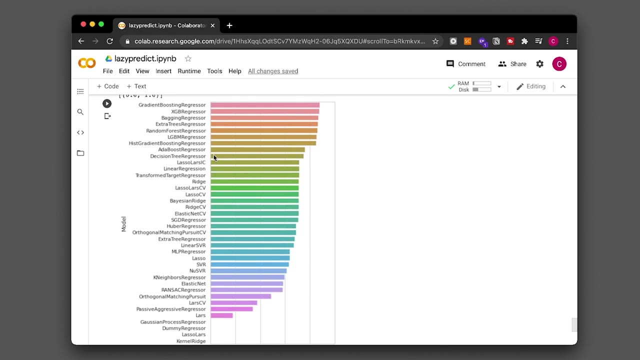 it would probably take you quite some time importing all of the libraries and then individually building it And then then aggregating the prediction results. so that would take a couple of hours to do. and so the lazy predict library allows you to build a default machine learning models by default. i mean they're 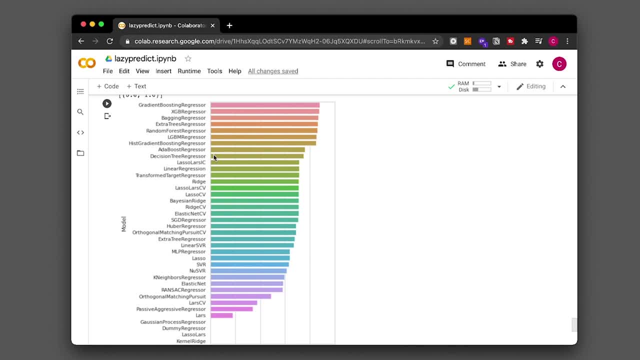 using default parameters. so the thing is, you cannot optimize the parameters here. you're just going to be building several machine learning models at the same time using the default parameters, which is still good because you're able to quickly build it- and then, once you identify which one is the best, then you focus your effort in performing hyper parameter optimization. for